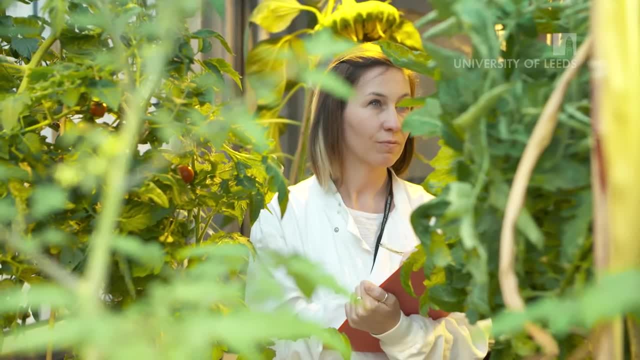 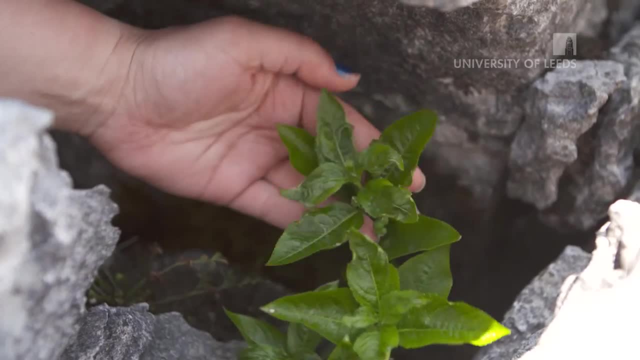 take the MSc or the MRes flavour of the Masters course. they'll be doing one or two substantial pieces of research which allow them to pursue their own interests and develop skills that they're interested in. Well, we try to provide our students with a long list of potential projects. 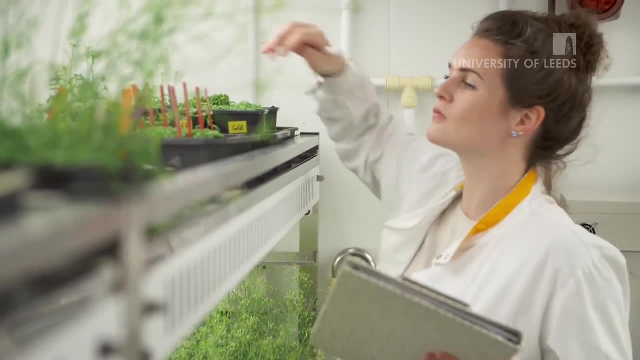 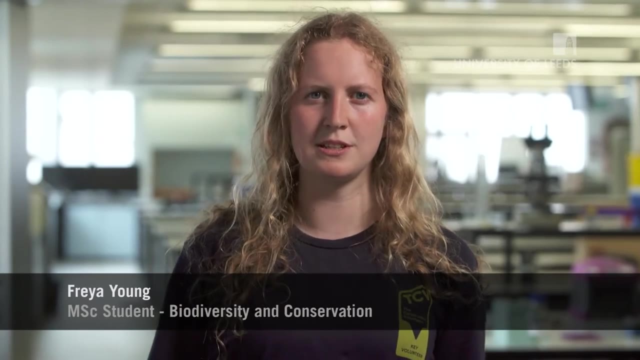 Which reflects the skills, experience and world leading research carried out by my colleagues and myself. I'm doing an MRes, which means I've got two research projects to do, So it's a research Masters. So I spent two months out in the Philippines, which was great and really interesting. 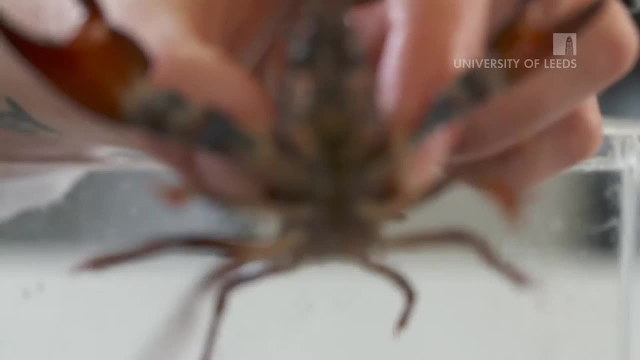 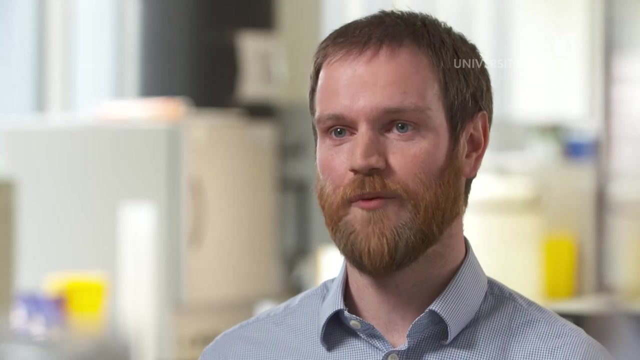 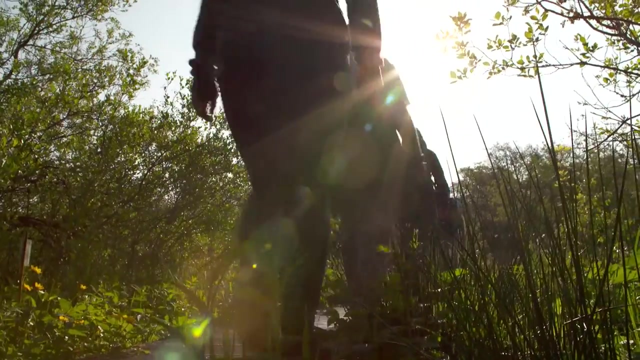 I was looking at physics- Big wasps. Other ones are things which external organisations have requested to us. They're, you know, for plant life or for natural England. It can be anything from lab based conservation, genetics analyses, through to social sciences and educational projects looking at how people in nature interact. 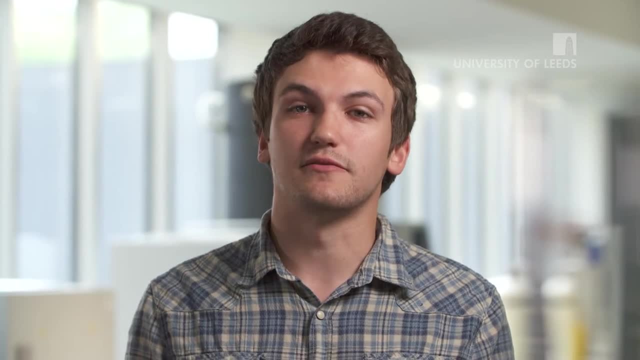 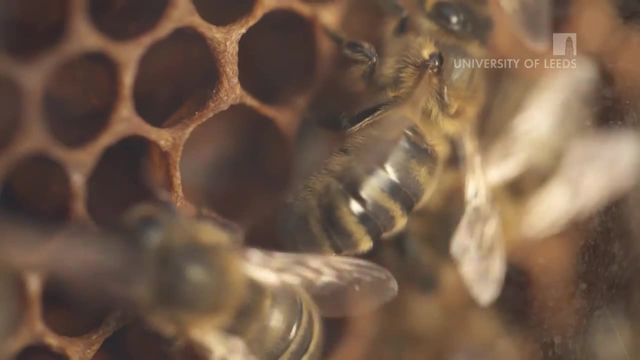 I approached one of the academics and he was at a meeting with the Beekeepers Association at that point- and he actually emailed me back and said: oh yeah, I think I can get you a project involving this Straight away. I was on that project. I was excited to start. 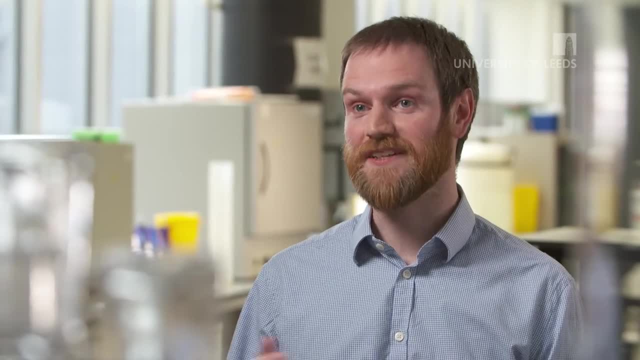 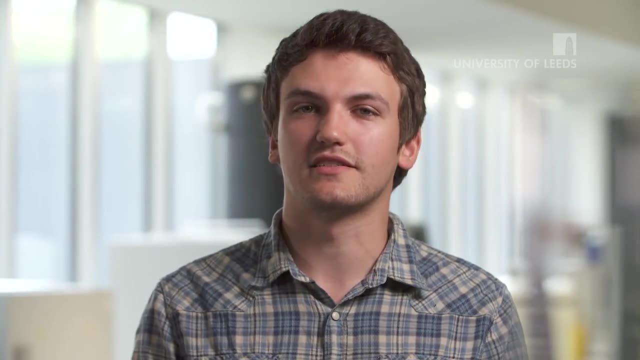 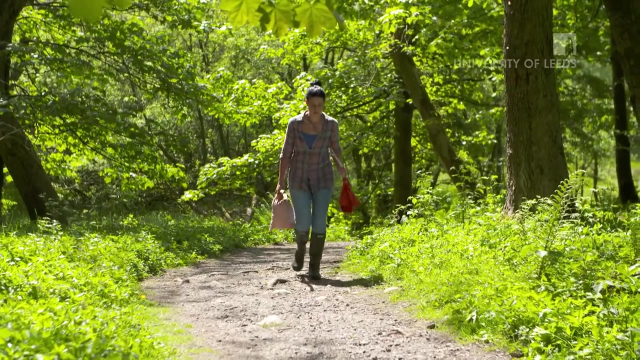 Often the students themselves are leading these research projects, or at least subsets of the projects, and contributing to some really innovative and unique ideas. I didn't expect to have such an interesting project that I can be so hands on with. It is hard work. They need to like being outdoors because there's a lot of outdoor work both. 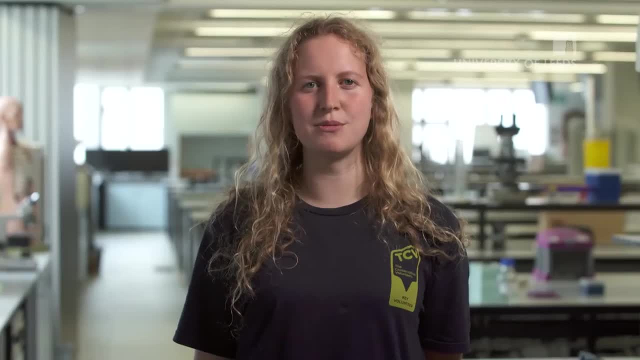 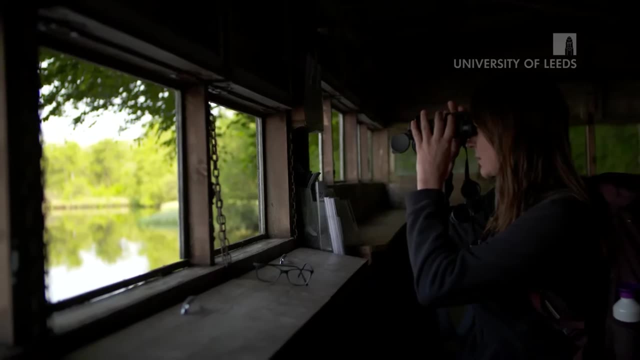 in the practical sessions and the modules and also in the field courses. The first thing we did was a sort of just a fairly casual get-to-know-each-other trip where we went and did some basic fieldwork skills up in Malham Tarn. 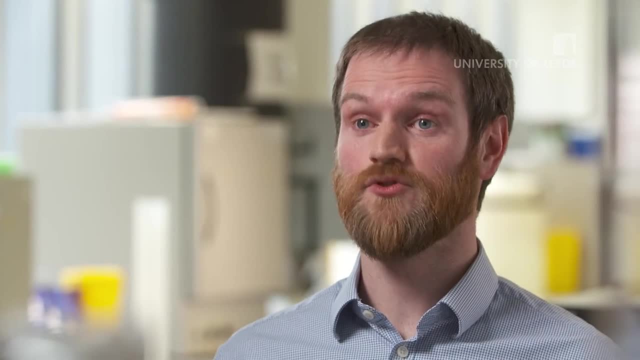 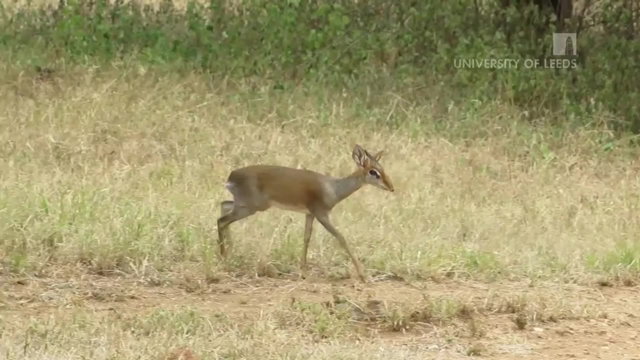 We run a course down to southern Spain, where the students experience one of the driest, the most arid areas of Europe. And then the most recent one that I've been on is the Africa field course. So we went to Kenya for two weeks. So we were driving around all day, every day, looking at different 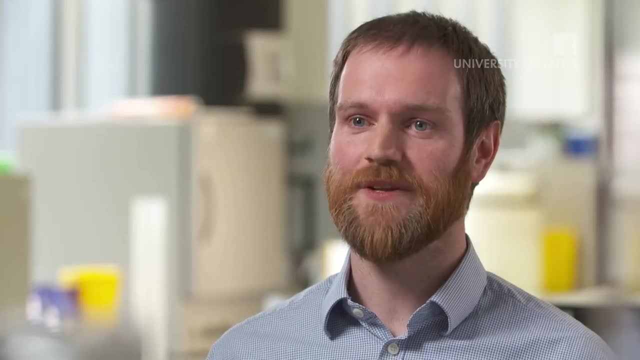 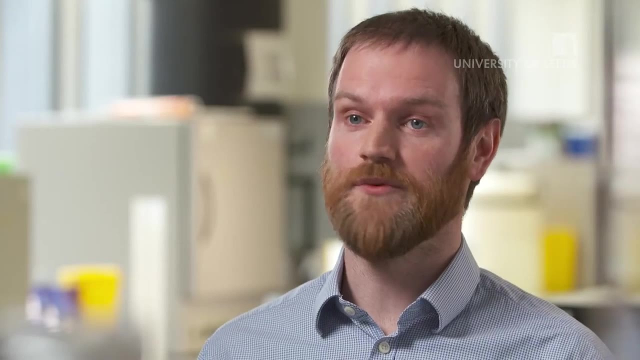 animals and taking down data on them. They get to understand what it means to conserve these valuable animals and see the cutting-edge research that goes on not only on those animals within the reserves that they visit, but also the slightly less charismatic animals, the ants and the plant communities that support.